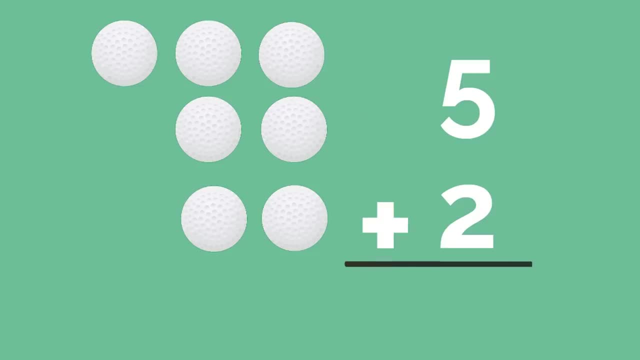 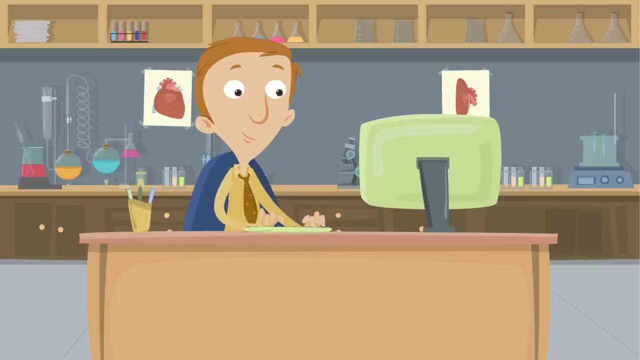 golf balls to the five that she already has. Remember. addition is putting numbers together together. Five plus two equals what? Here's a hint: You can count these golf balls up and get the answer: Yeah, seven. Five plus two equals seven. You are doing a tremendous. 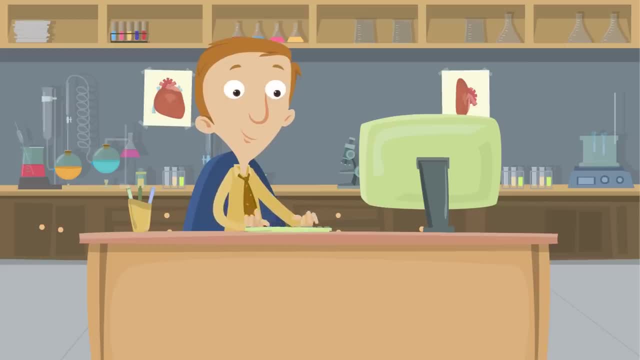 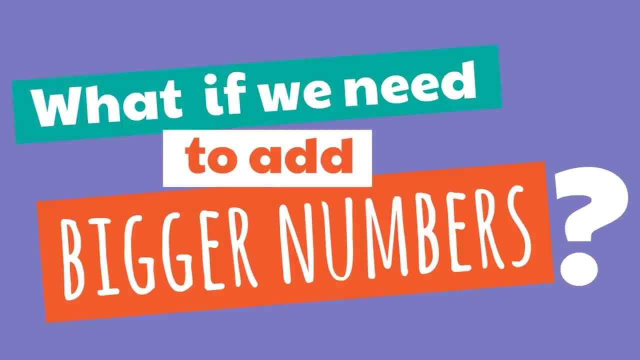 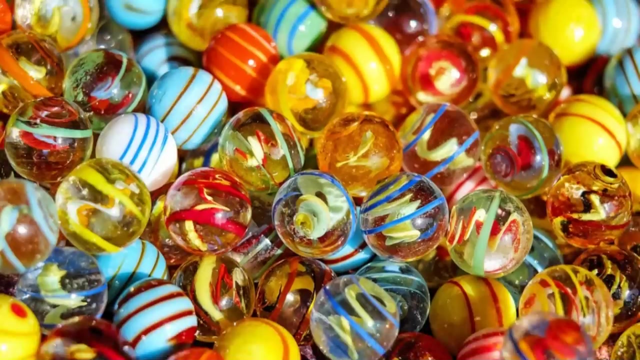 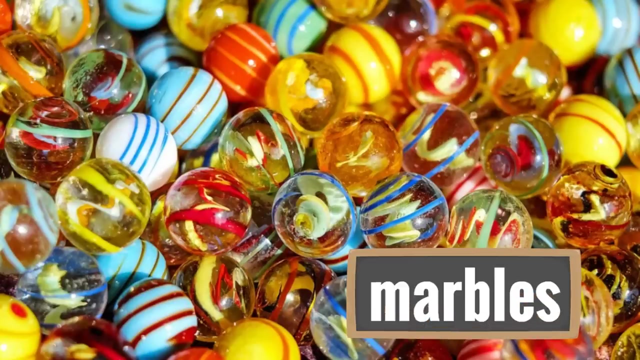 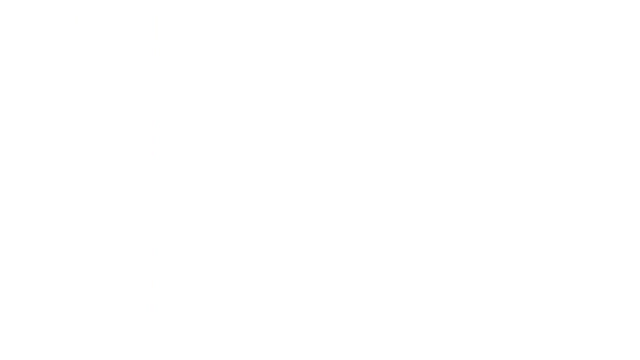 job. These are examples of single digit addition. But what if we need to add bigger numbers? Yeah, Let's say there's this kid named Travis. Hi, Travis, Travis collects these. What are these called? Uh-huh, Marbles Travis collects marbles Travis had a lot of marbles He had. 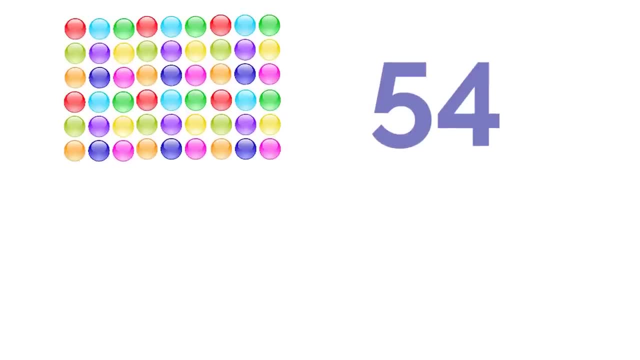 54 marbles, But today is his birthday and someone just gave him 21 more marbles. Wow. Now he wants to know: how many marbles do I have? I had 54 and now I have 21 more that are in my collection. How many marbles do I have? That's the question that Travis has. 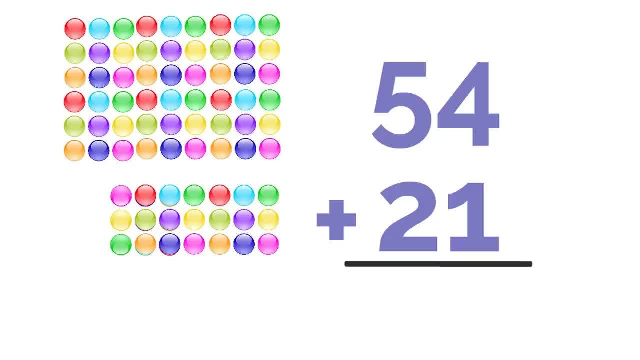 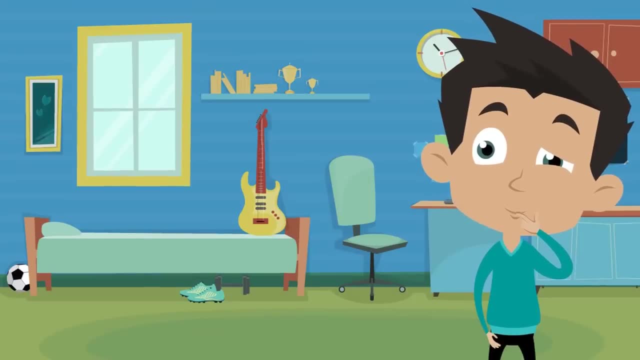 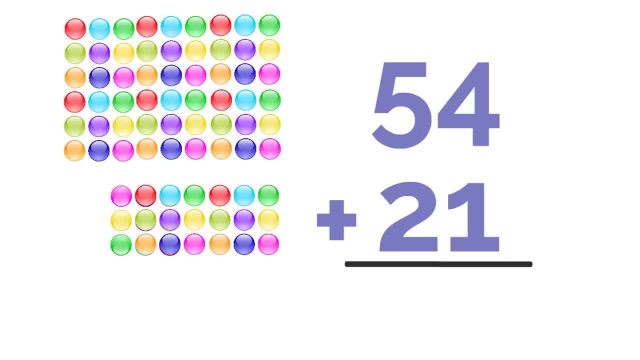 marbles do I have now? Now you should start thinking of how many marbles have you added that you have added? I don't think you question too much about how many marbles you have. longer time. Look at these marbles. The way that you can add lots of them has an issue. Look at each. 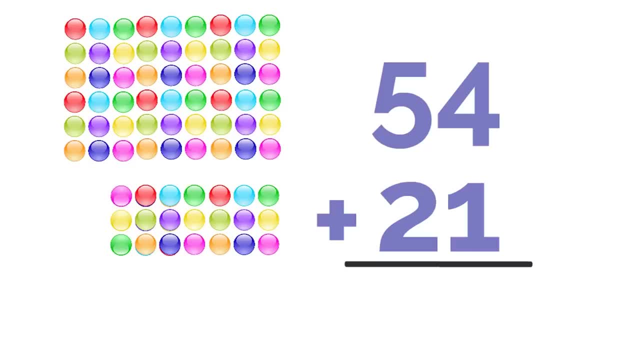 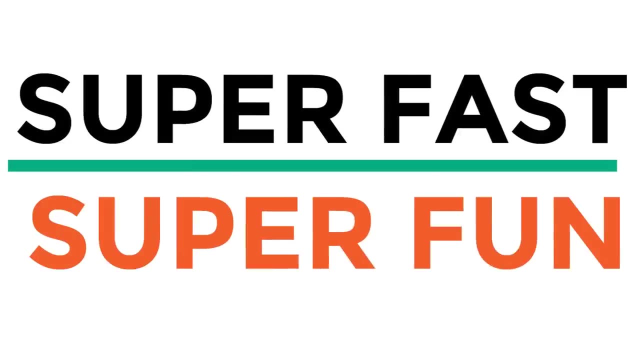 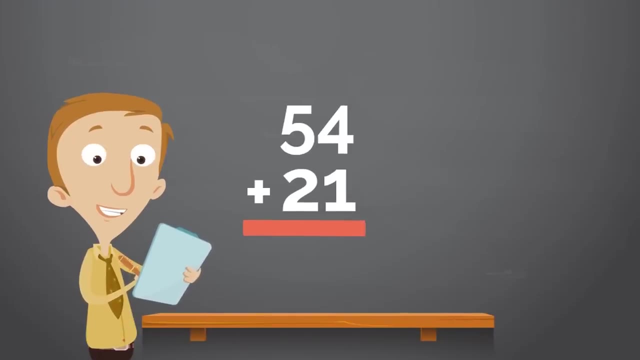 of these marbles. Look at each of these marbles. There has to be a better way. in fact there is. There's a way that is super fast and super fun. How many of these marbles can be added? We can add 54 and 21 together. by doing a fun trick, We'll turn these big numbers that 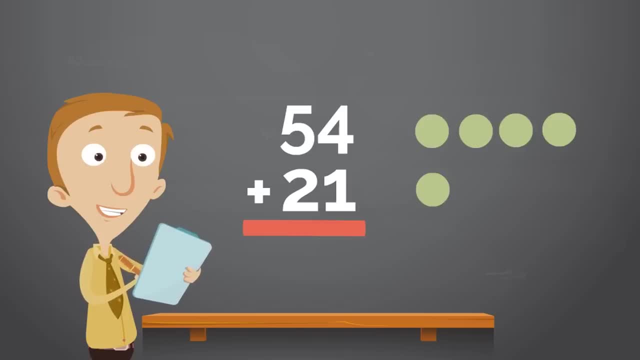 are difficult to add on their own into smaller numbers. What you will do is you will add the numbers to the right, right here, which are the ones to make it easier. we are going to block the 10 spot for right now with this nifty blue rectangle. suddenly this huge, big addition problem. 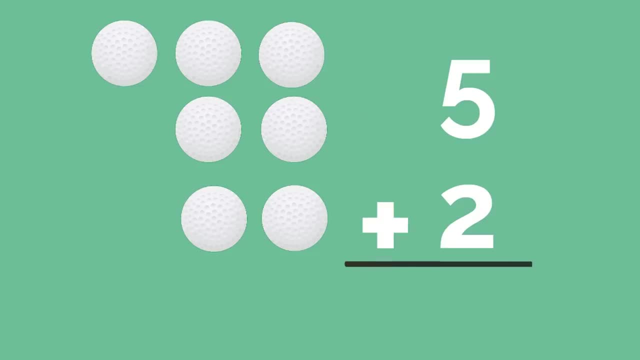 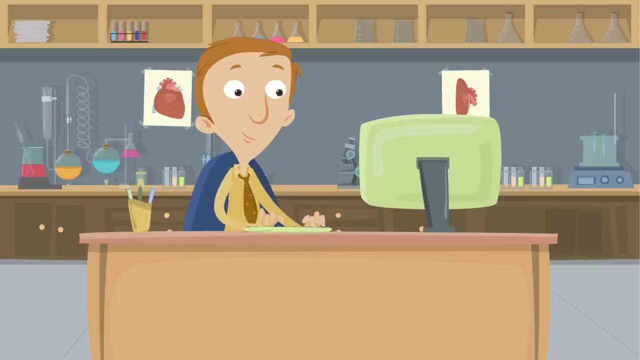 golf balls to the five that she already has. Remember. addition is putting numbers together together. Five plus two equals what? Here's a hint: You can count these golf balls up and get the answer: Yeah, seven. Five plus two equals seven. You are doing a tremendous. 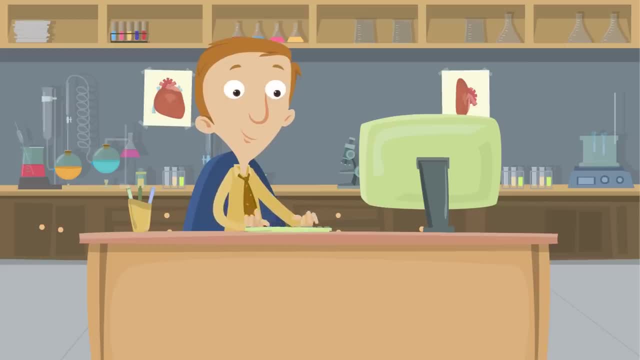 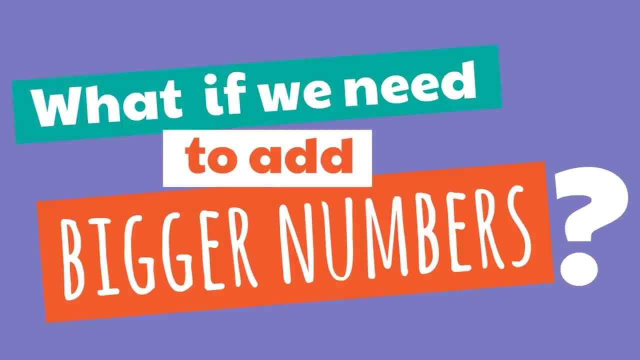 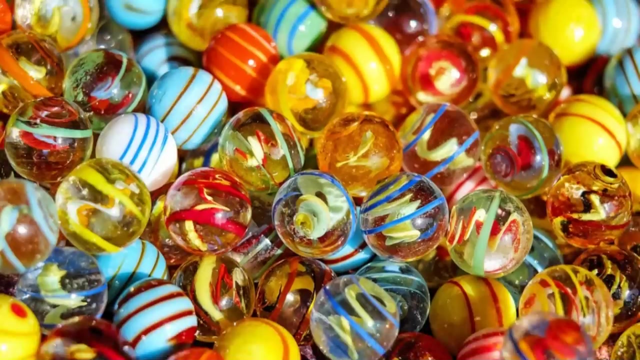 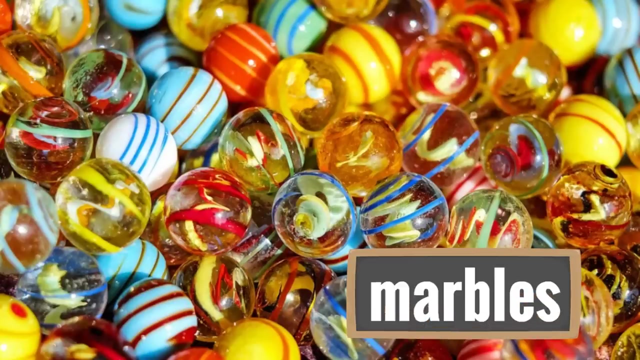 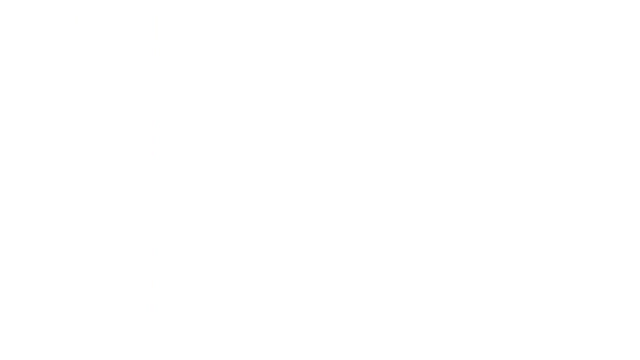 job. These are examples of single digit addition. But what if we need to add bigger numbers? Yeah, Let's say there's this kid named Travis. Hi, Travis, Travis collects these. What are these called? Uh-huh, Marbles Travis collects marbles Travis had a lot of marbles He had. 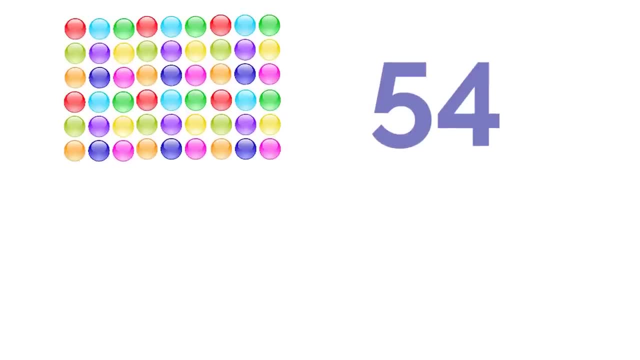 54 marbles, But today is his birthday and someone just gave him 21 more marbles. Wow. Now he wants to know: how many marbles do I have? I had 54 and now I have 21 more that are in my collection. How many marbles do I have? That's the question that Travis has. 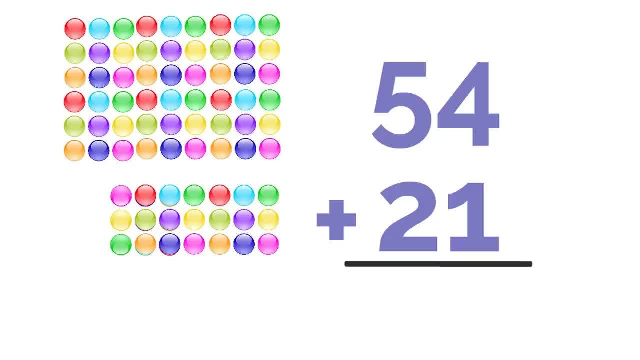 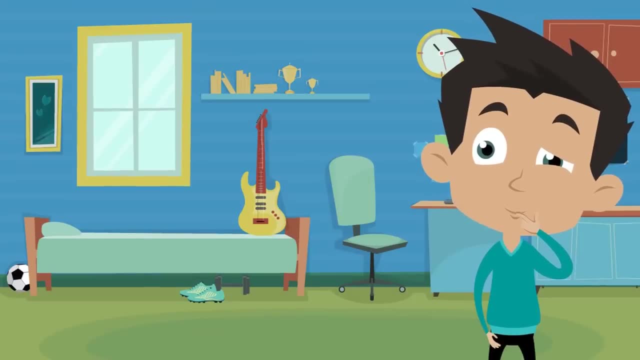 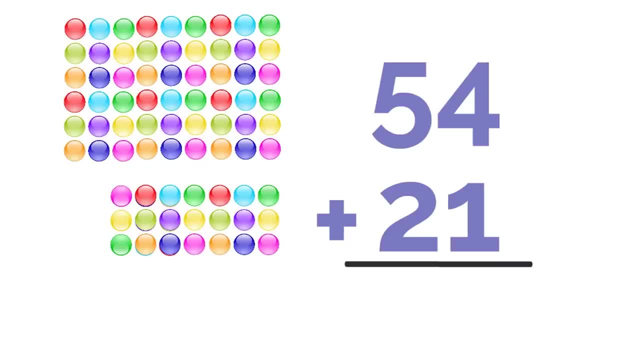 marbles do I have? How many marbles do I have? How many marbles do I have? How many of these marbles? There has to be a better way. In fact there is. There's a way that is super fast. 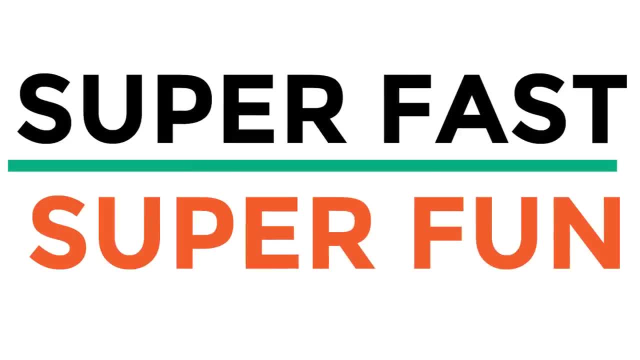 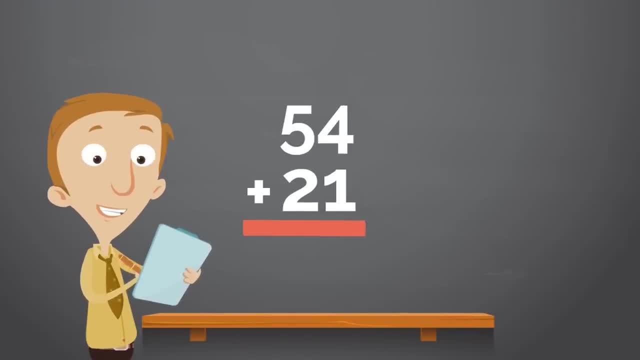 and super fun. We can add 54 and 21 together. by doing a fun trick, We'll turn these big numbers that are difficult to add on their own into smaller numbers. What you will do is you will add the numbers to the right right here, which are the ones To make it easier. we are going to 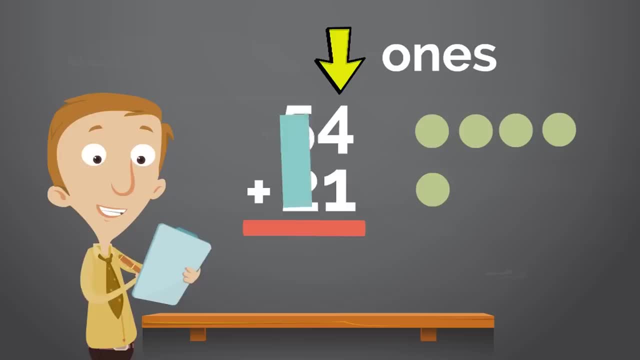 block the 10 spot for right now with this nifty blue rectangle. Suddenly, this huge big addition problem has turned into a simple fun addition game. So we add the right spot, the one spot together. What is 4 plus 1?? Hmm, Yes, 4 plus 1 equals 5.. So we'll write 5 under the 4 and the. 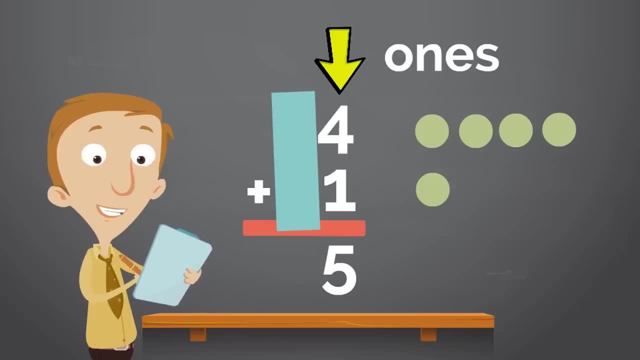 1. Awesome job, We're halfway done already. 5, 5. Next we will add the 10s together. The 10 spot is to the left. The 2 numbers in the 10 spot are the 5 and 2.. To make it easier, we are going to block the 1 spot with another blue rectangle. 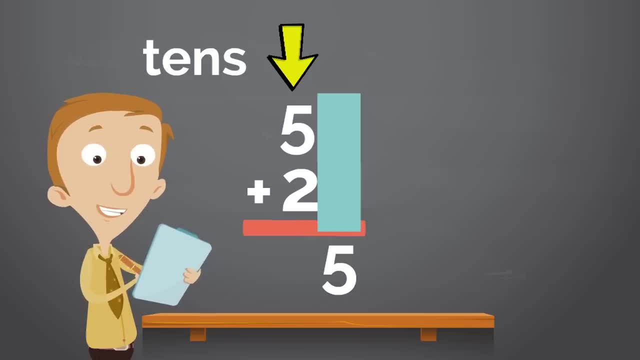 because we already added the 1 spot up. What is 5 plus 2?? Uh-huh, 5 plus 2 equals 7.. So we will write 7 under the 5 and the 2.. So what is our answer? What is 54 plus 21?? Uh-huh, You can see it right here: 75.. 54 plus 21 equals 75.. 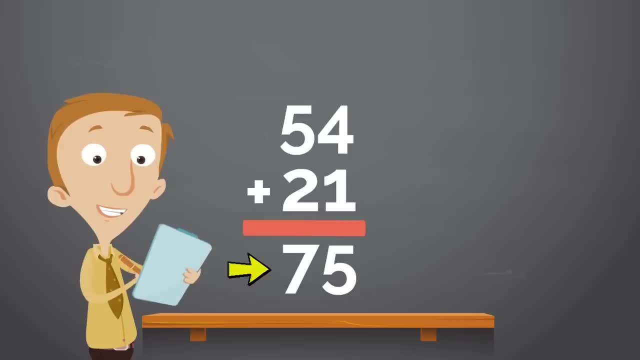 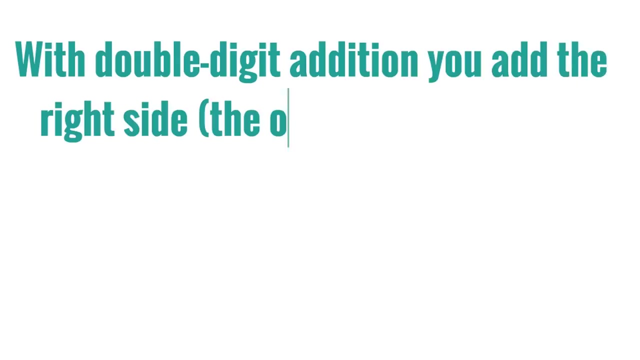 The answer to an addition problem is called the sum. Our sum is 75. It's simple: With double digit addition we will add 2. Addition: you add the right side, the ones together. first Let's figure out what 30 plus 12 is. first. 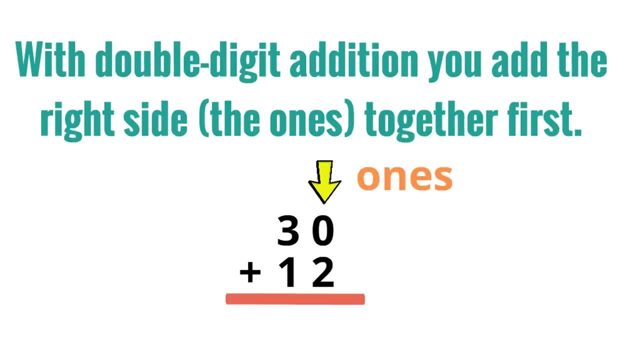 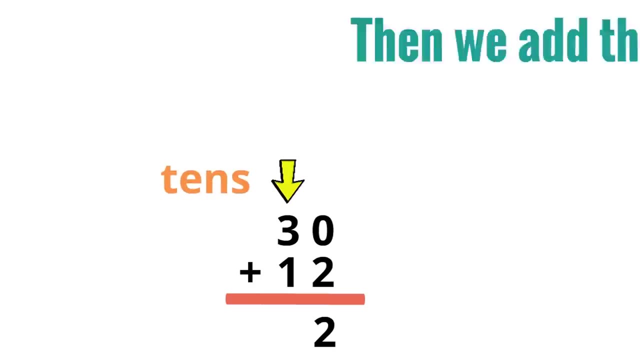 What is 0 plus 2?? Yes, 0 plus 2 is 2, so we'll write a 2 under the right side, the one side. We've almost arrived at our answer already. Then we add the left side, the tens, to get our answer. what is 1 plus 3? 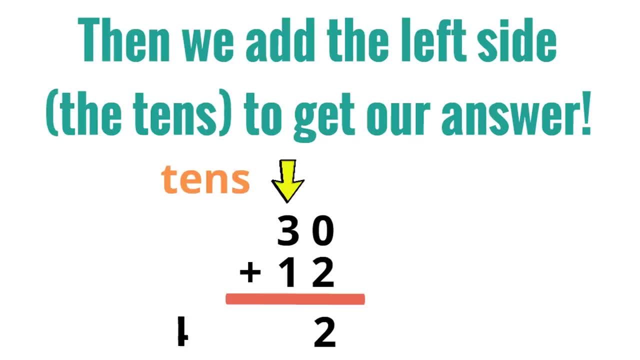 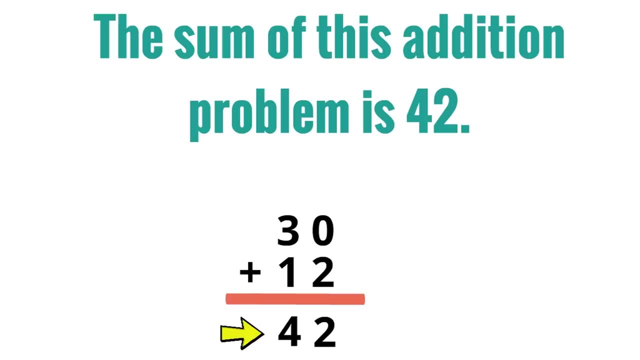 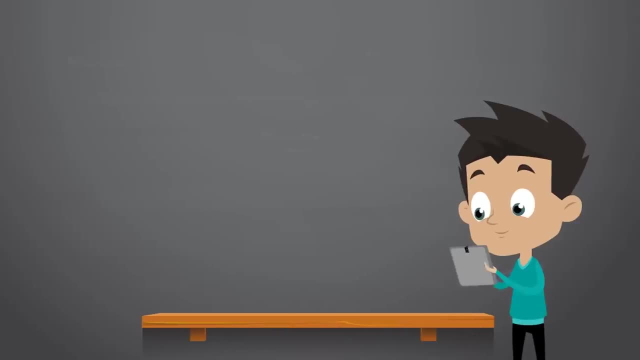 Yep: 1 plus 3 equals 4, So the sum of this addition problem is 42. 30 plus 12 equals 42. Let's try a different type of addition problem: 33 plus 6. this is an interesting one, because 33 is a double-digit number. 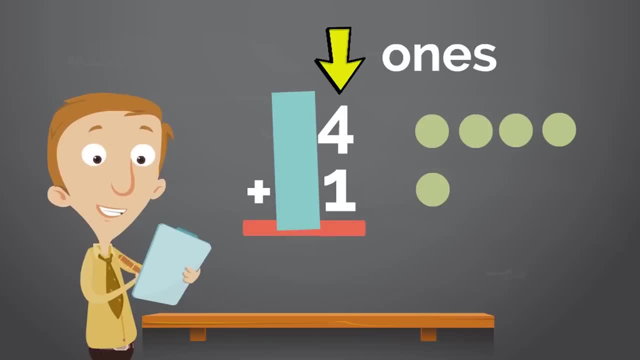 has turned into a simple fun addition game. so we add the right spot, the one spot together. what is 4 plus 1? yes, 4 plus 1 equals 5, so we'll write 5 under the 4 and the 1. awesome job, we're halfway. 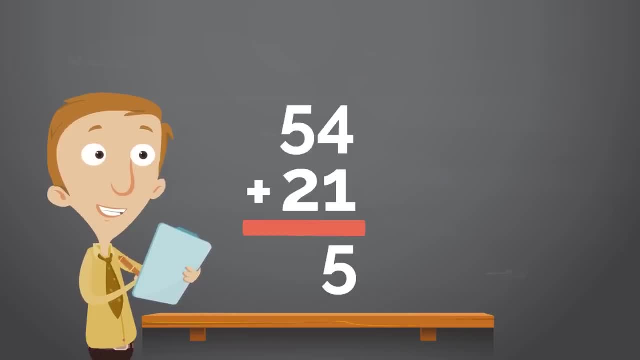 done already. next we will add the 10s together. the 10 spot is to the left. the two numbers in the 10 spot are the 5 and 2. to make it easier, we are going to block the one spot with another blue rectangle, because 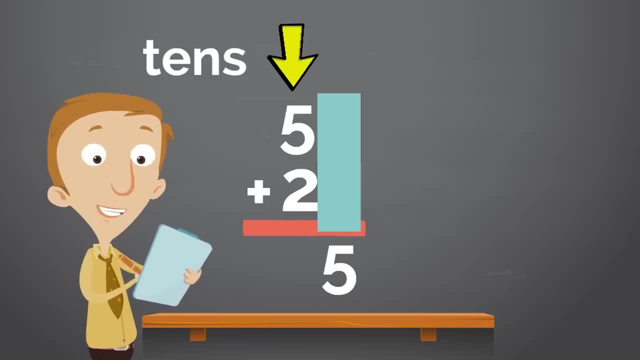 we already added the one spot up. What is 5 plus 2?? Uh-huh, 5 plus 2 equals 7.. So we will write 7 under the 5 and the 2.. So what is our answer? What is 54 plus 21?? Uh-huh, You can see it right. 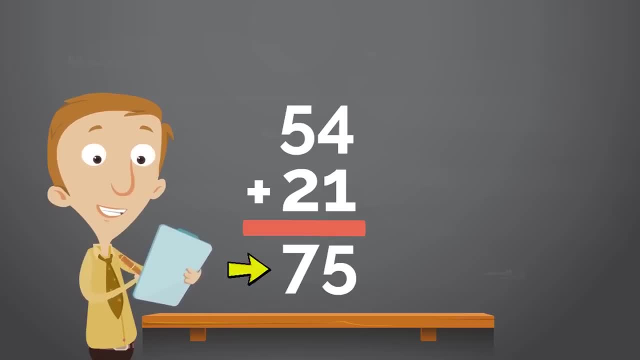 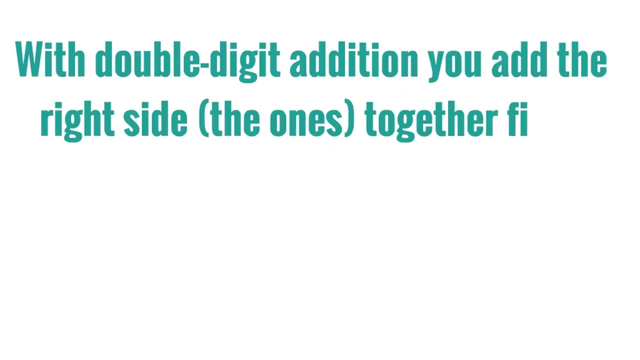 here 75.. 54 plus 21 equals 75.. The answer to an addition problem is called the sum. Our sum is 75.. It's simple With double digit addition. you add the right side, the ones together first. 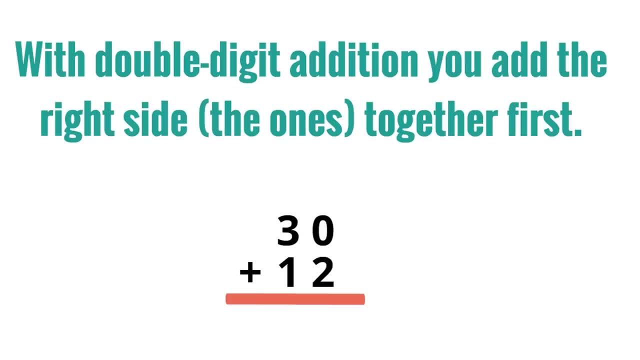 Let's figure out what 30 plus 12 is First. what is 0 plus 2?? Yes, 0 plus 2 is 2.. So we'll write a 2 under the right side, the ones side. We've almost arrived at our answer already. Then we add the left side. 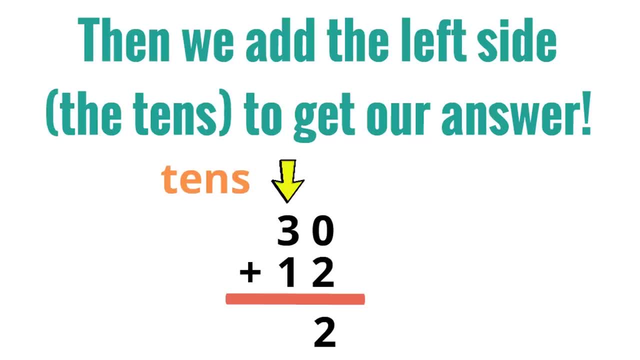 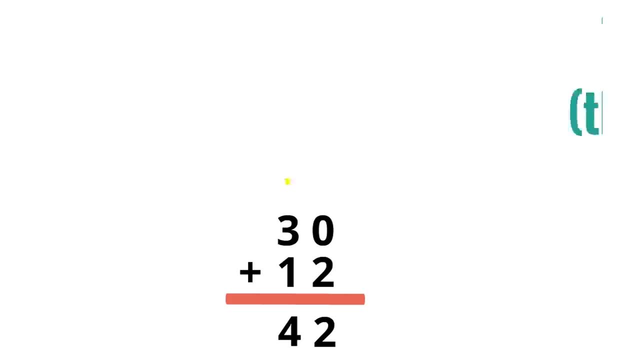 the tens to get our answer. What is 1 plus 3?? Yep, 1 plus 3 equals 4.. So the answer to an addition problem is called the sum. What is 1 plus 2?? Uh-huh, You can see it right. 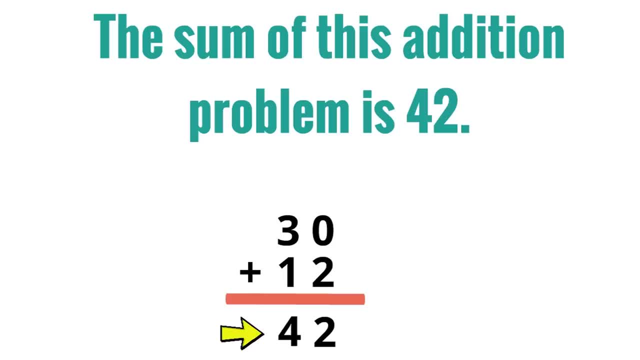 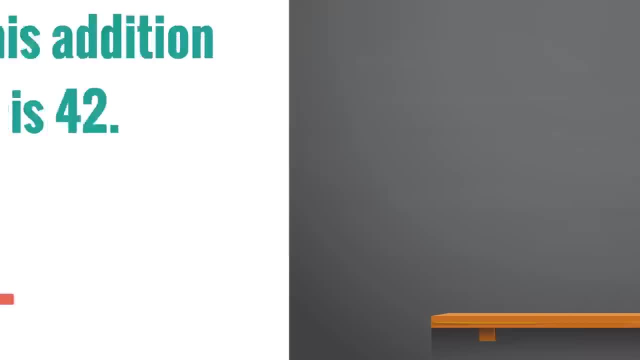 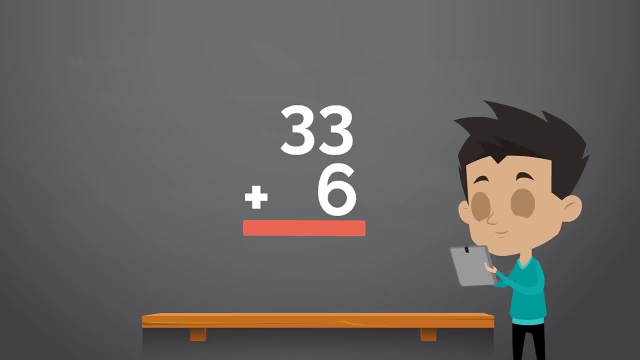 here. So the sum of this addition problem is 42.. 30 plus 12 equals 42.. Let's try a different type of addition problem: 33 plus 6.. This is an interesting one, because 33 is a double digit number, but the 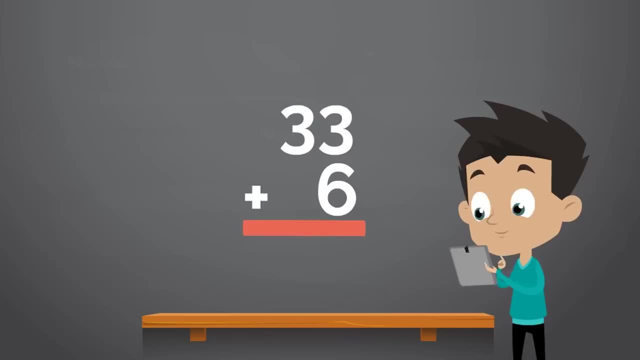 But the number 6 is a 6. It's a single-digit number, but we use the same fun trick as before. First we add up the ones. What is 3 plus 6?? hmm, uh-huh, 3 plus 6 equals 9. so we write 9 here under the ones. 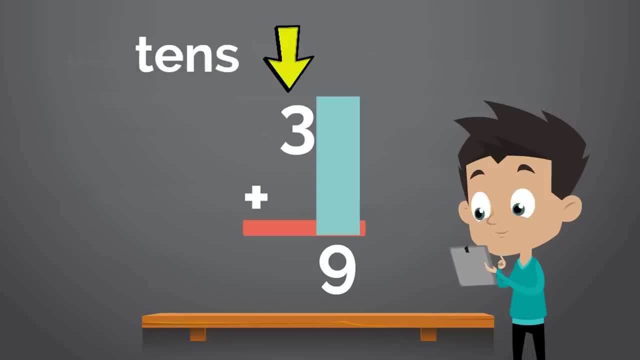 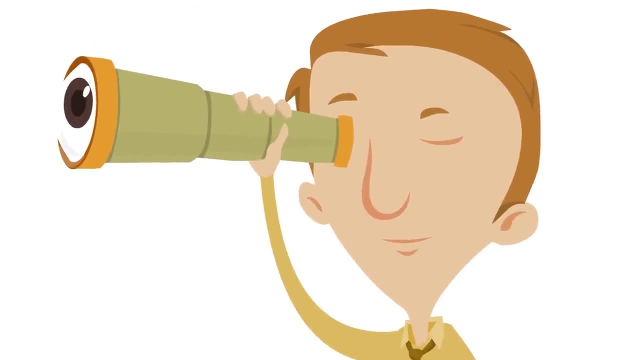 Next, let's add up the tens. but there is only one number in the ten spot. So what do you get If you add nothing to 3? Uh-huh, you get 3. So what is our sum? yes, our sum is 39. How are we doing? 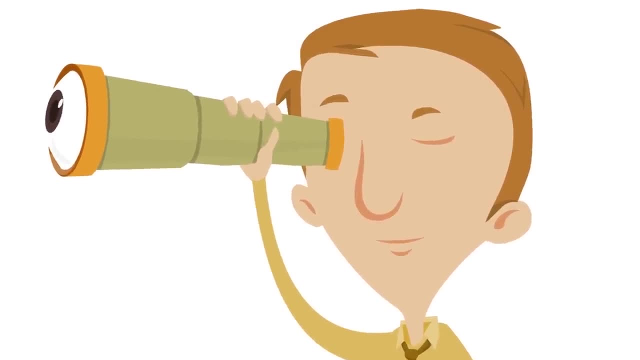 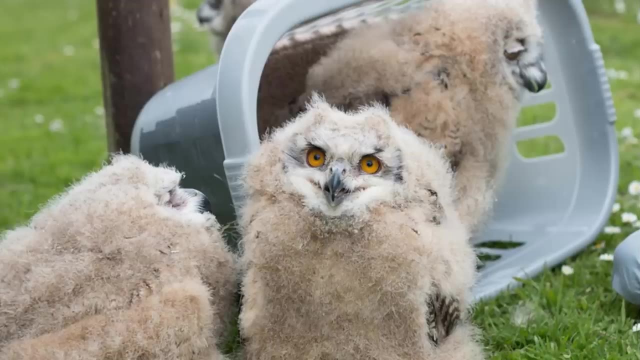 Double-digit addition is pretty cool, isn't it? Now we are going to talk about something special, really special. Special like seeing an owlette, a little bird, a little baby owl looking at you, looking at your eyes, so cute, so special. so what is this special? 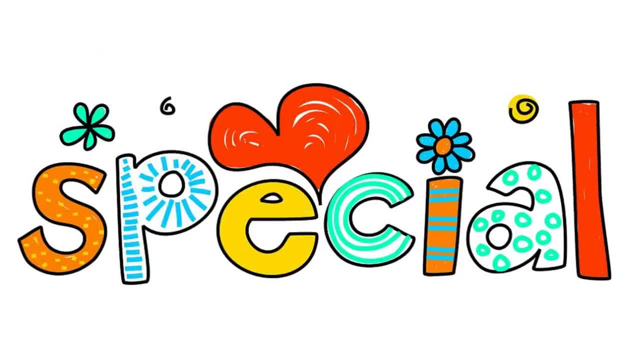 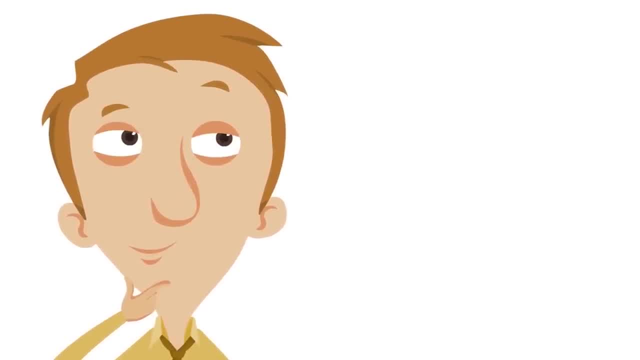 thing we are about to learn. well, sometimes something sneaky happens. let's show you. let's say we are adding 17 plus 15. we of course start with the right side, adding up the ones first. so what is 7 plus 5? do you know? 7 plus 5? yeah, 7 plus 5 equals 12, that's right, but there's only. 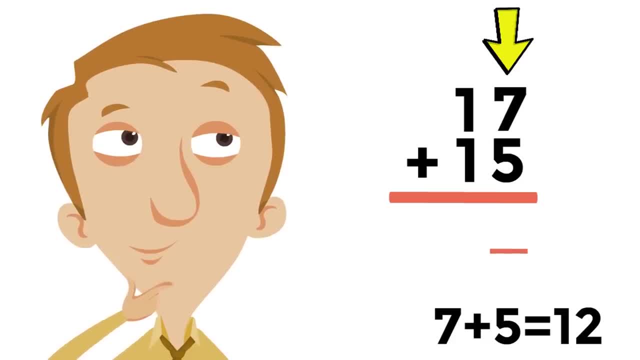 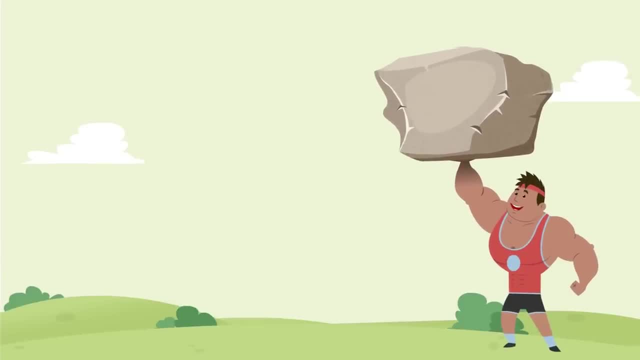 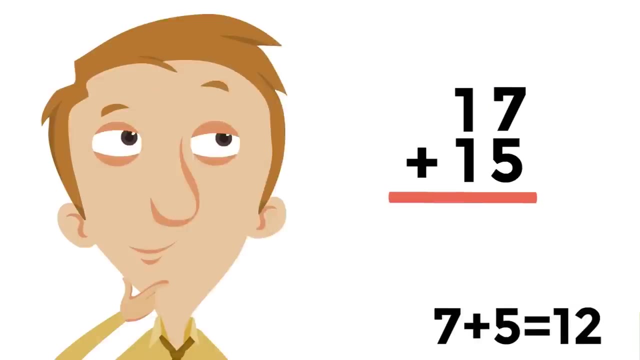 enough room for one digit under the 7 and the 5. so what do you do? well, we do a super cool move called regrouping, regrouping, regrouping is awesome. remember the sum of our ones column is 12. 7 plus 5 equals 12. so we have to regroup the number 12. but 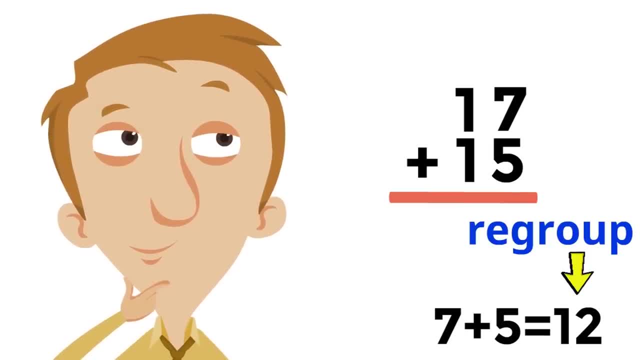 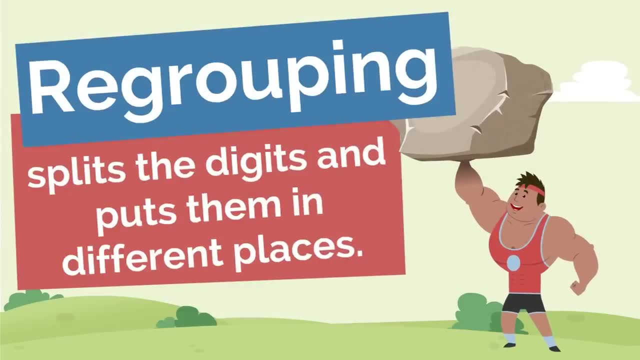 what does that mean? what does regrouping even do? well, regrouping splits the digits and puts them in different places. now that might sound weird, but we're going to show you how it works. it's super simple and fun regrouping the number 12. 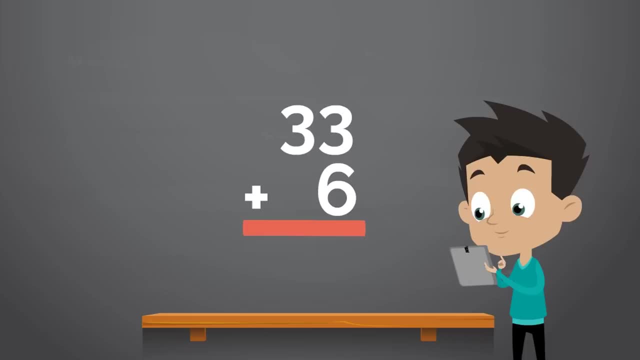 number 6 is a single digit number, But we use the same fun trick as before. First we add the add up the ones. What is 3 plus 6?? Hmm, Uh-huh, 3 plus 6 equals 9.. So we write 9 here under the ones. 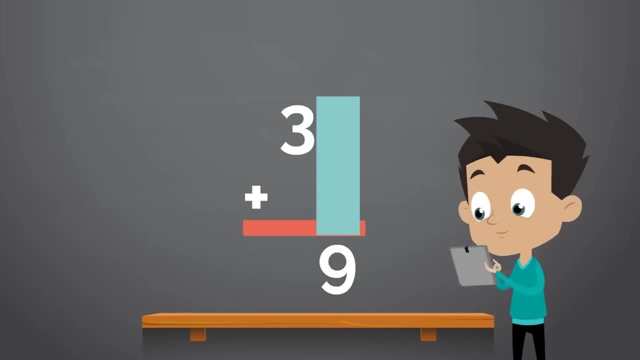 Next, let's add up the tens. but there is only one number in the tens spot. So what do you get if you add nothing to 3?? Uh-huh, You get 3.. So what is our sum? Yes, our sum is 39.. 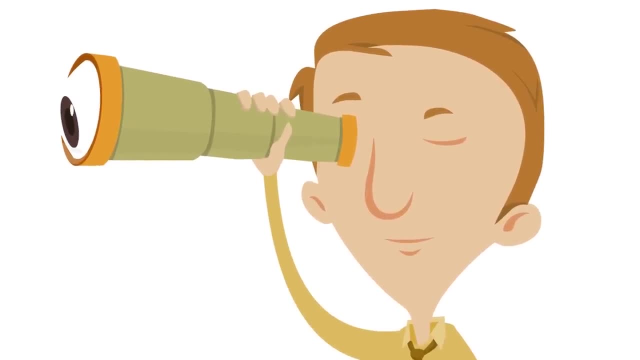 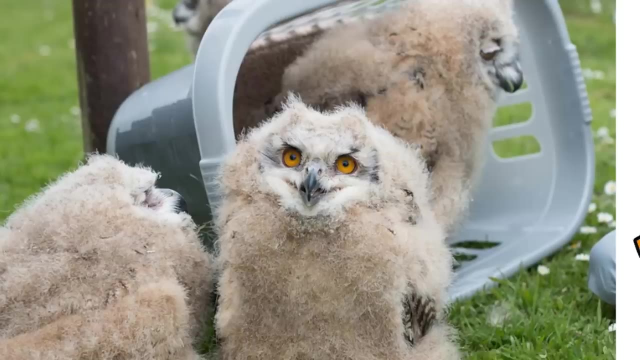 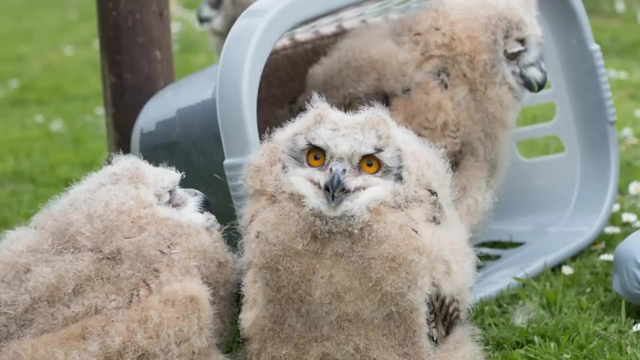 How are we doing? Double digit edition is pretty cool, isn't it? Now we are going to talk about something special, Really special. Special, like seeing an owlette, a little baby owl, looking at you, looking at your eyes, So cute, so special. 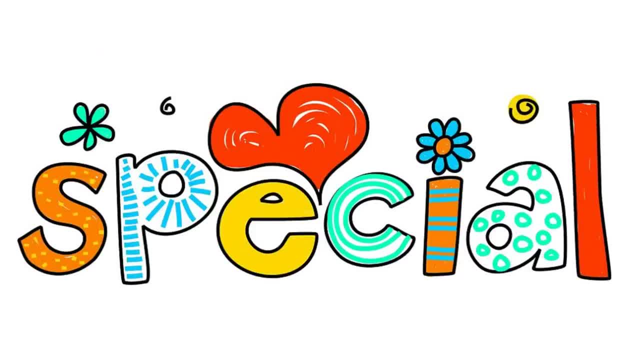 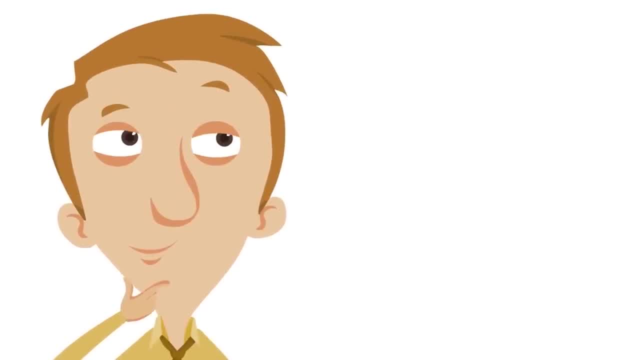 So what is this special thing we are about to learn? Well, sometimes something sneaky happens. Let's show you. Let's say, we are adding 17 plus 15.. We, of course, start with the right side, adding up the ones first. 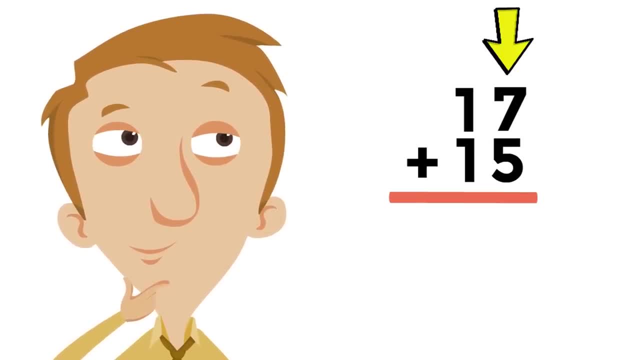 So what is 7 plus 5?? Do you know 7 plus 5.? Yeah, 7 plus 5.. 7 plus 5 equals 12.. That's right, But there is only enough room for one digit under the 7 and the 5.. 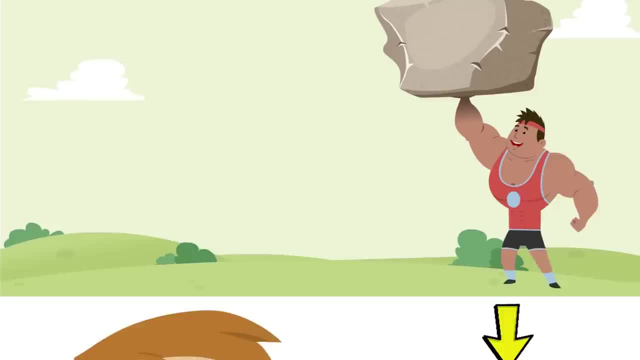 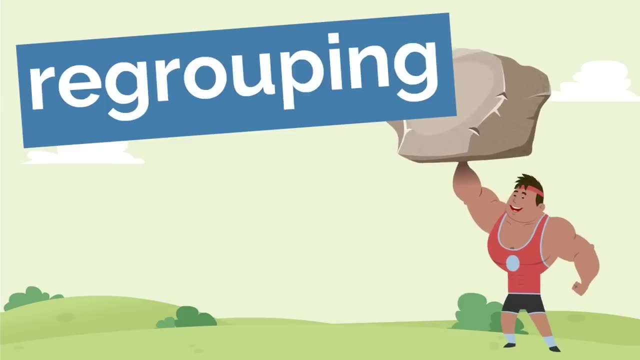 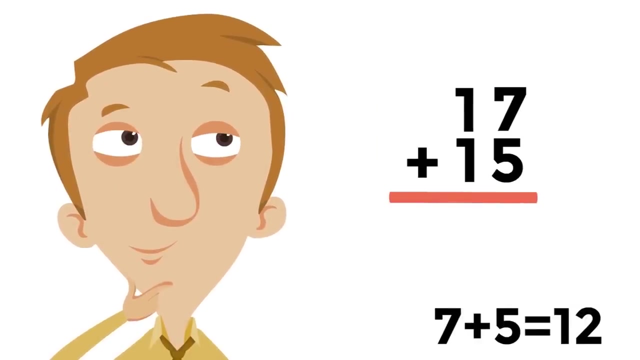 So what do you do? Well, we do a super cool move called regrouping, Regrouping, Regrouping is awesome. Remember the sum of our ones column is 12.. 7 plus 5 equals 12.. 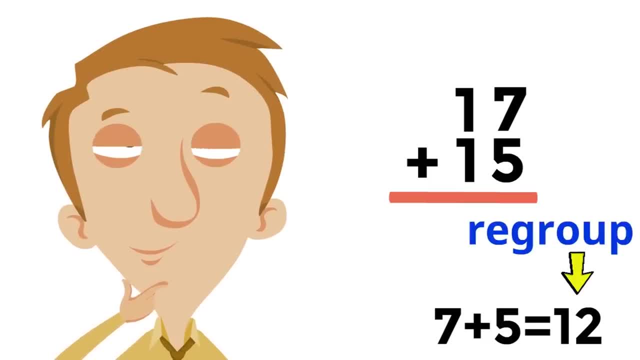 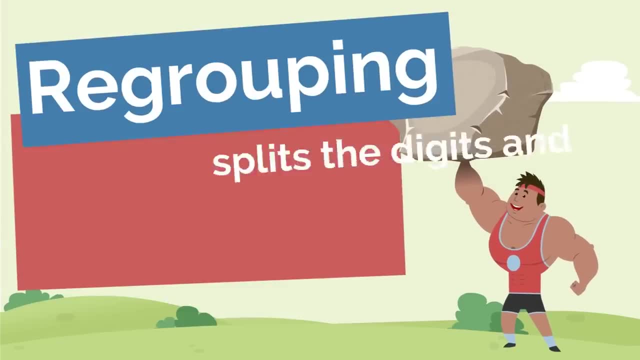 So we have to regroup the number 12.. But what does that mean? What does regrouping even do? Well, regrouping splits the digits and puts them in different places. Now, that might sound weird, but we are going to show you how it works. 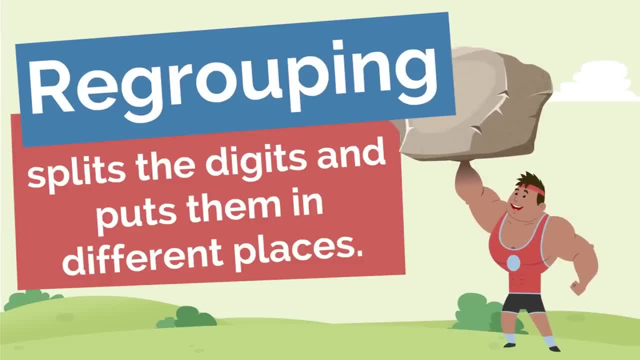 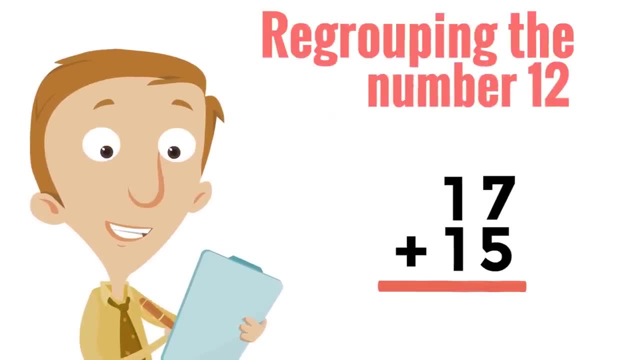 It's super simple and fun. Regrouping the number 12 is easy. All we do is split the digits, putting the 2 under the ones and carrying the 1 with the 10s. That's it. Then we add up the 10s. 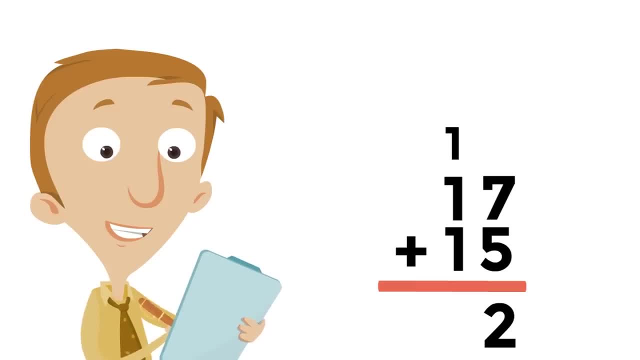 What is 1 plus 1 plus 1?? Yeah, 1 plus 1 plus 1 equals 3.. So we write 3 under the 10s And now we have our answer: 17 plus 15 equals 32.. 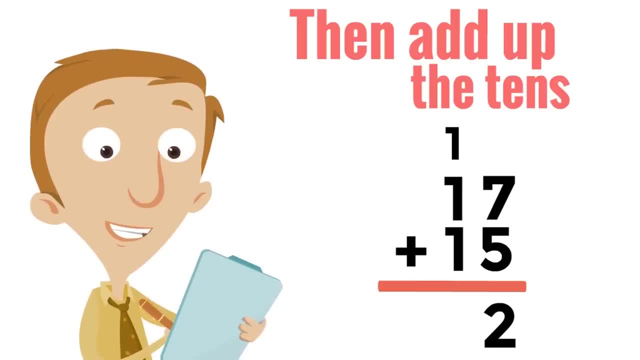 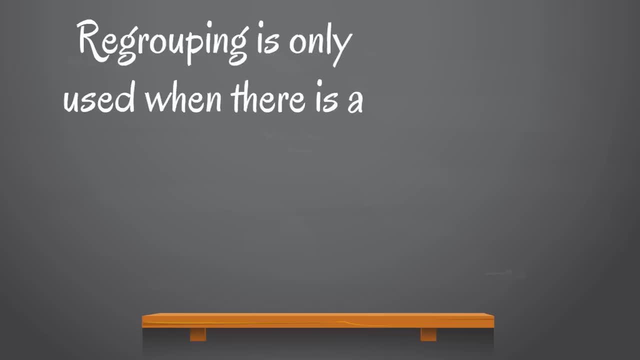 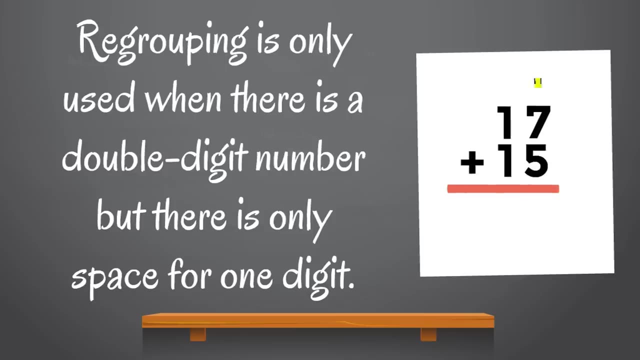 Remember, regrouping is only used when there is a double digit number, but there is only space for one digit. Like our example: 7 plus 5 equals 12.. But there wasn't enough room for both numbers, So we keep the 2 under the ones and carry the 1 to the 10s. 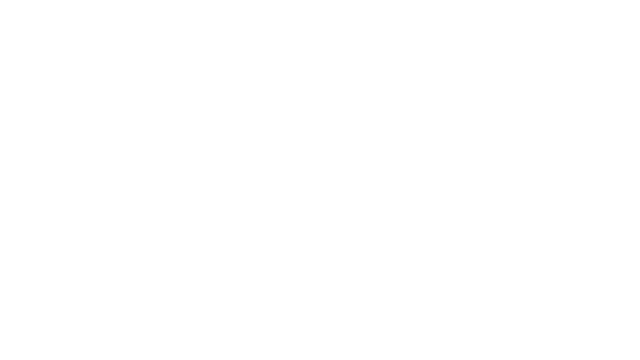 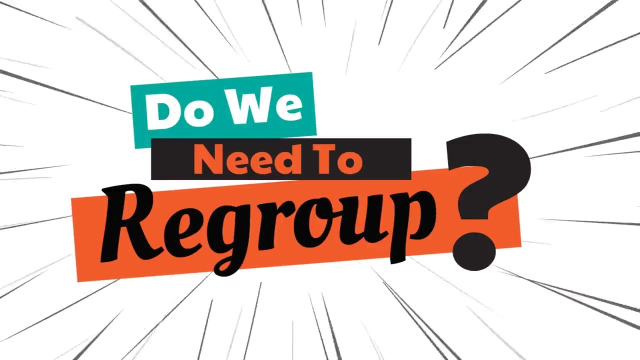 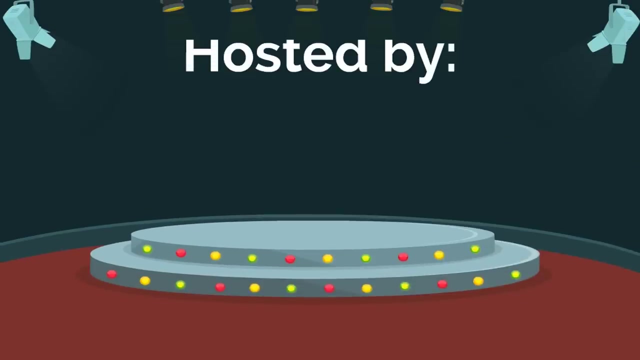 Hey, let's practice by playing a game. The game is called: Do We Need to Regroup? This is probably the most exciting double digit edition game ever Hosted by our very own Mr Whiskers. Thanks for helping our show. 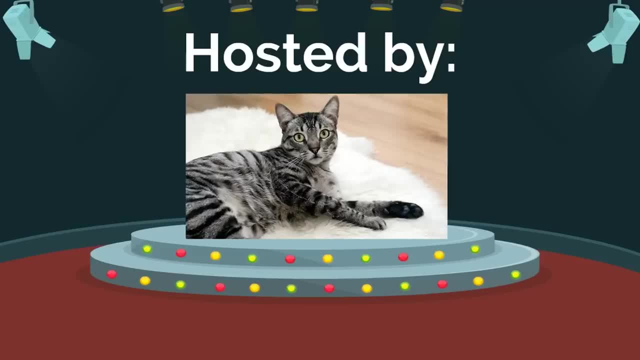 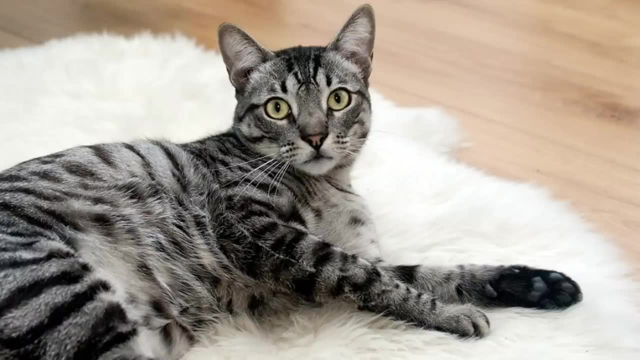 You're not going to help us out. Okay, Okay, now this is embarrassing. Okay, Fine, Okay, Alright, That's okay, That's alright, That's alright, It's okay, It's okay, Alright. Well, we are going to look at double digit edition problems. 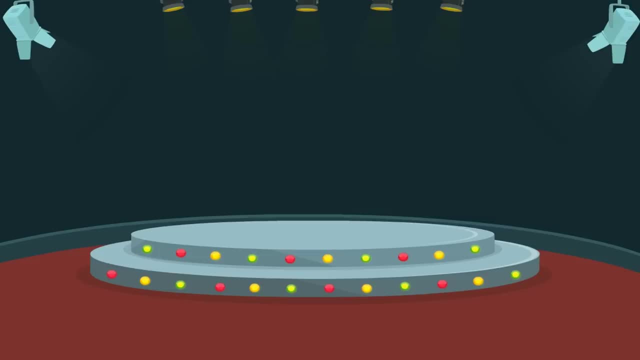 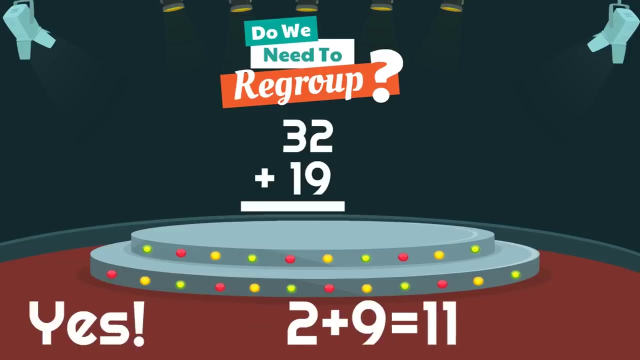 And you are going to let us know. Do we need to regroup? Here is our first problem: 32 plus 19.. You already know the question: When we add 32 and 19, do we need to regroup? Yes, because 2 plus 9 equals 11,, which is a double digit number. 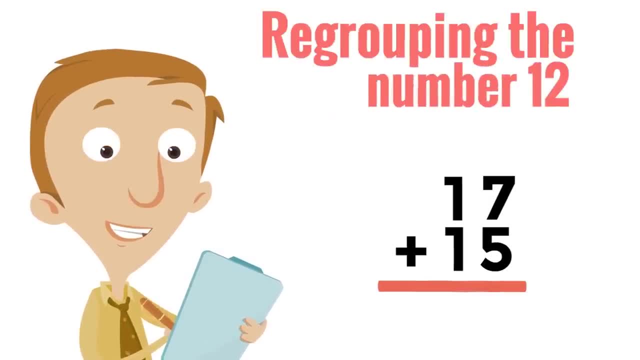 typically, this way is easy. all we do is split the digits, putting the two under the ones and carrying the one with the tens up here. that's it. then we add up the tens. what is one plus one plus one? 1 plus 1 plus 1 equals 3. so we write 3 under the tens and now we have our 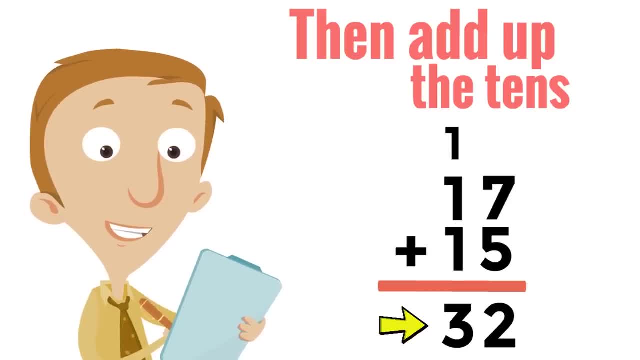 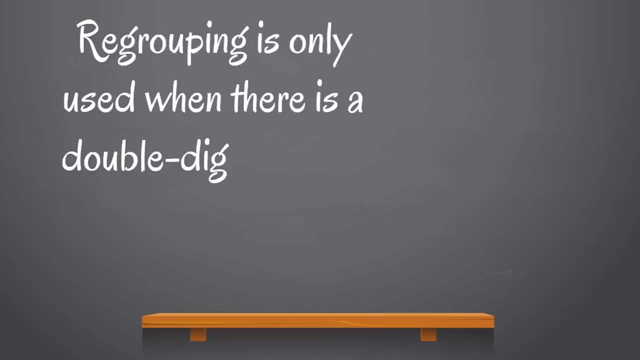 answer: 17 plus 3, 15 equals 32.. 32 is our sum. Remember, regrouping is only used when there is a double-digit number, but there is only space for one digit, Like our example. 7 plus 5 equals 12.. 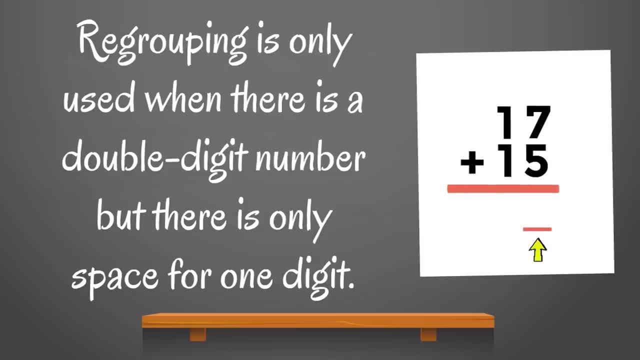 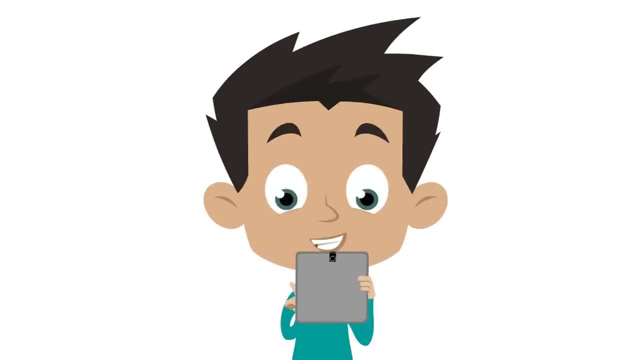 But there wasn't enough room for both numbers, so we keep the 2 under the 1s and carry the 1 to the 10s. Hey, let's practice by playing a game. The game is called: Do We Need to Regroup? 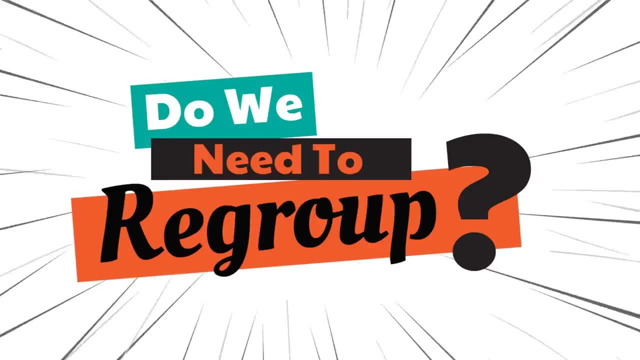 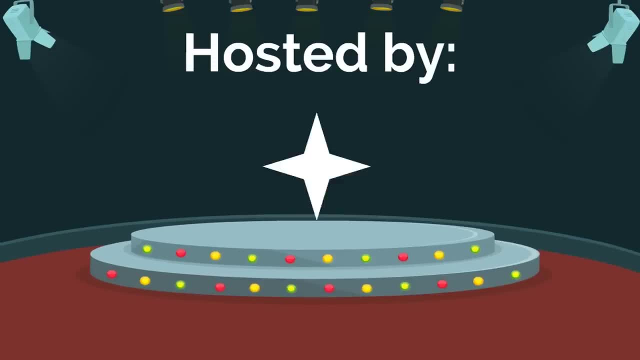 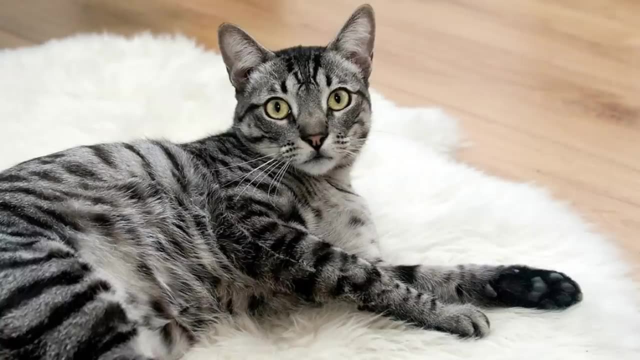 This is probably the most exciting double-digit edition game ever Hosted by our very own Mr Whiskers. Thanks for helping us out. You're not going to help us out, Okay, Okay, now, Now, this is embarrassing, Okay. 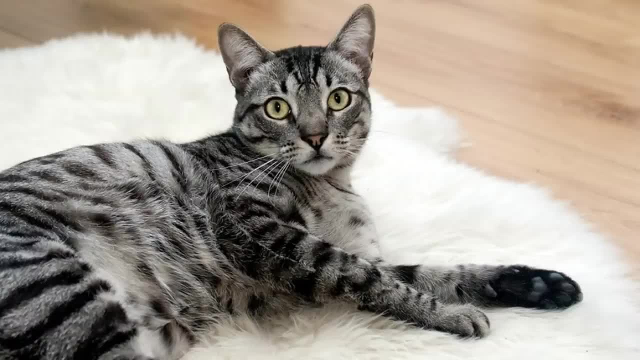 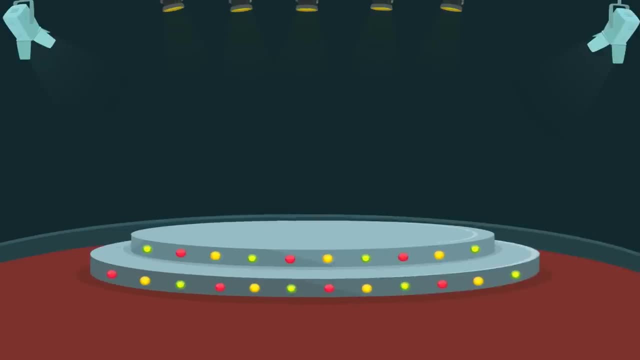 Fine, Okay, Alright, That's okay, That's alright, That's alright. Okay, That's okay, Alright. Well, we are going to look at double-digit edition problems and you are going to let us know. Do we need to regroup? 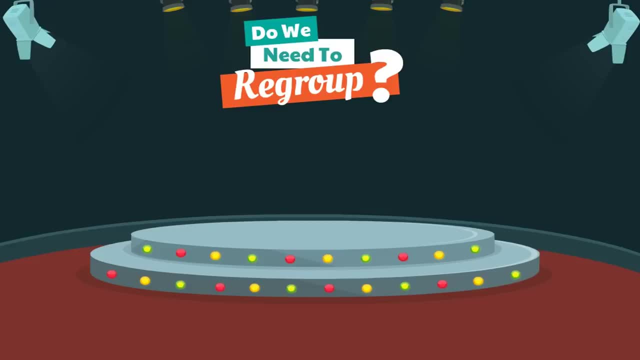 Here is our first problem: 32 plus 19.. You already know the question: When we add 32 and 19,, do we need to regroup? Yes, because 2 plus 9 equals 11,, which is a double-digit number. 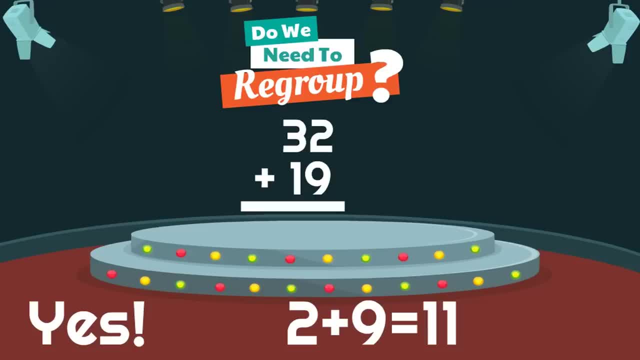 Remember, the first step we take is adding up the 1s, But if the sum is a double-digit number, that means we need to regroup. Great job, Let's go ahead and finish the problem. When we regroup, we split the digits. 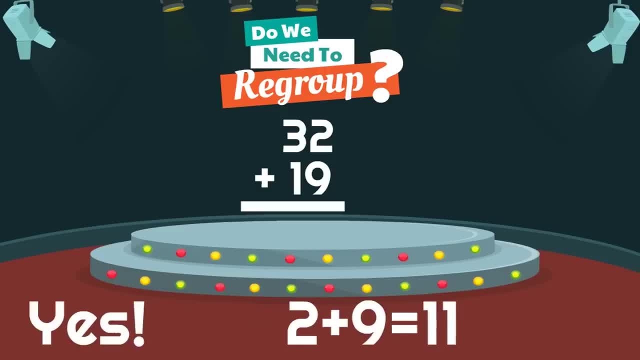 Remember, the first step we take is adding up the ones, But if the sum is a double digit number, that means we need to regroup. Great job, Let's go ahead and finish the problem. We regroup, We split the digits. 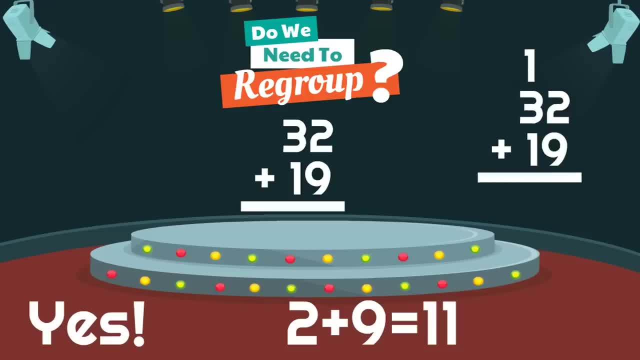 So the first one gets carried And the second number- in this case also the number 1, stays down under the ones. Then we just add up the tens. What is 1 plus 3 plus 1?? Uh-huh, 5.. 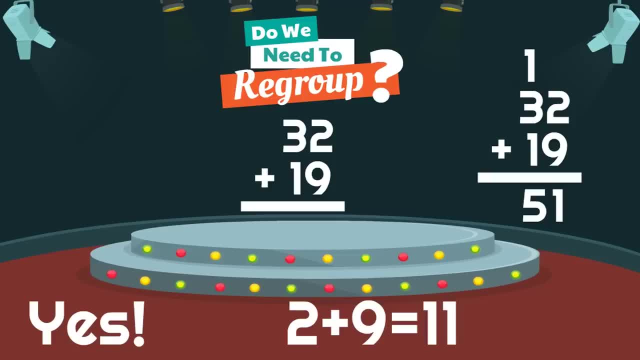 So 32 plus 19 equals 51. And yes, we did have to regroup. Here is our second one: 56 plus 22.. This is the question: When we add 56 and 22, do we need to regroup? 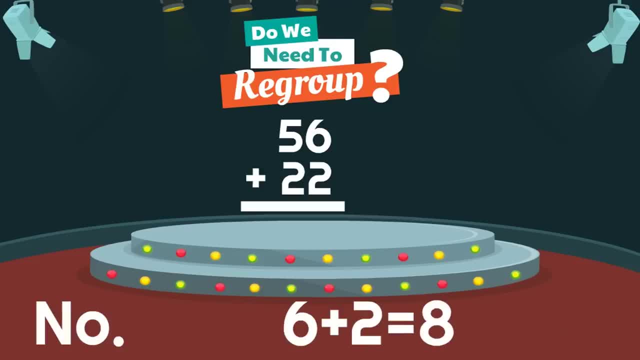 No, because 6 plus 2 equals 8.. And 8 is a single digit number that can fit under the ones. Remember, the first step we take is adding up the ones And since the sum is a single digit number already, we do not need to regroup. 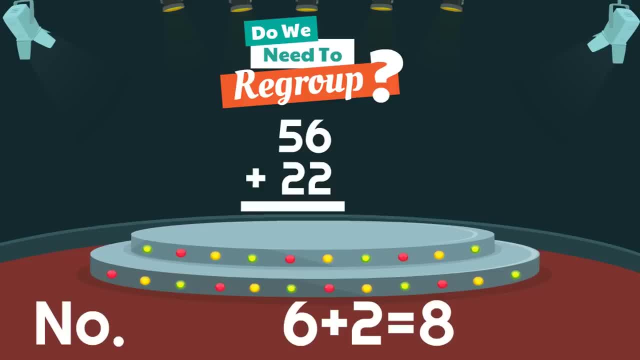 Fantastic, Let's go ahead and finish the problem. So when we added up the ones, our sum was 8.. We'll put the 8 under the ones. Then we just add up the tens. What is 5 plus 2?? 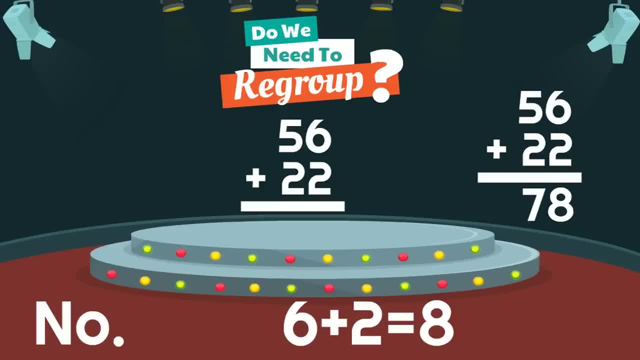 Uh-huh, 7.. And we have our answer: 56 plus 22 equals 78. And no, we did not have to regroup. Here is our next one: 34 plus 25.. This is the question: When we add 34 and 25, do we need to regroup? 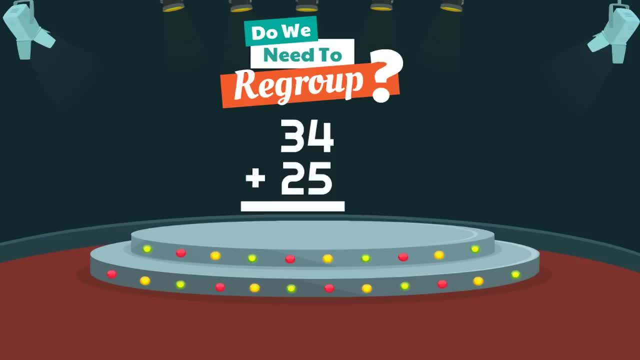 Yes, So how many to sits did we add? We added 2,, so 4 plus 3 equals 9.. And the answer is no, Because 4 plus 5 equals 9.. And 9 is a single digit number that can fit under the ones. 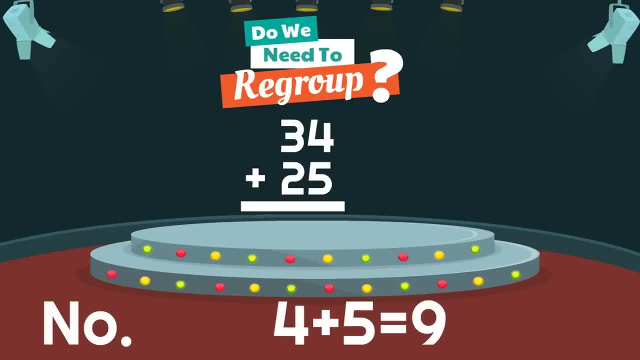 Remember, the first step we take is adding up the ones, And since the sum is a single digit number already, we do not need to regroup. Well done, Let's go ahead and finish the problem, just for fun. So when we added up the ones, our sum was 8.. 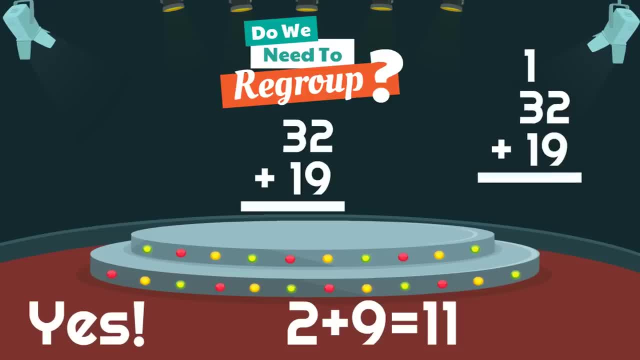 So the first 1 gets carried and the second number- in this case also the number 1, stays down under the 1s. Then we just add up the 10s. What is 1 plus 3 plus 1?? 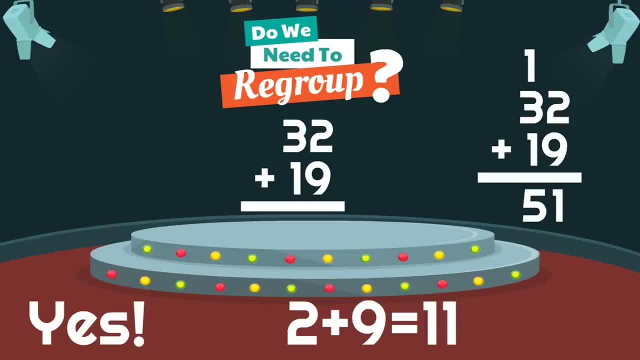 Uh-huh, 5.. So 32 plus 19 equals 1.. Uh-huh, 5 plus 19 equals 5.. And yes, we did have to regroup. Here is our second problem: 56 plus 22.. 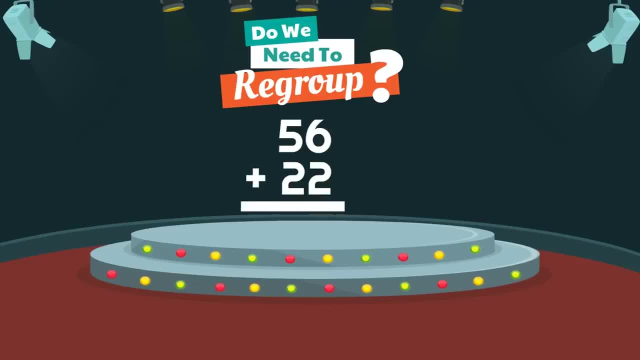 This is the question: When we add 56 and 22,, do we need to regroup? No, Because 6 plus 2 equals 8.. And 8 is a single-digit number that can fit under the 1s. Remember, the first step we take is adding up the 1s. 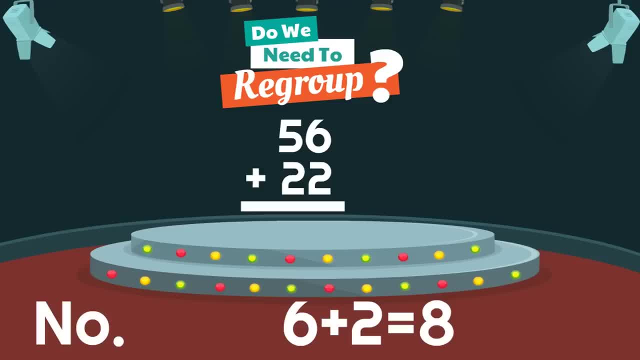 And since the sum is a single-digit number already, we do not need to regroup Fantastic. Let's go ahead and finish the problem. So when we added up the 1s, our sum was 8.. We'll put the 8 under the 1s. 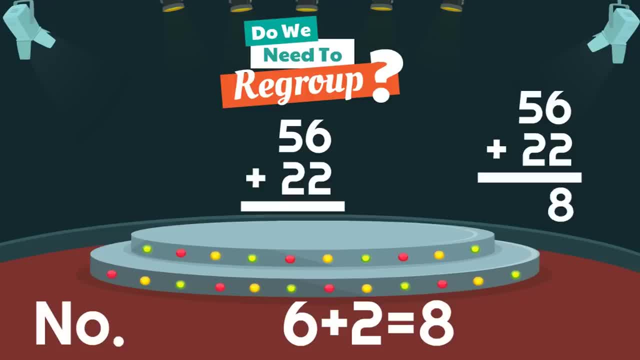 Then we just add up the 10s. What is 5 plus 2?? Uh-huh, 7.. And we have our answer: 56 plus 22 equals 78. And no, we did not have to regroup. 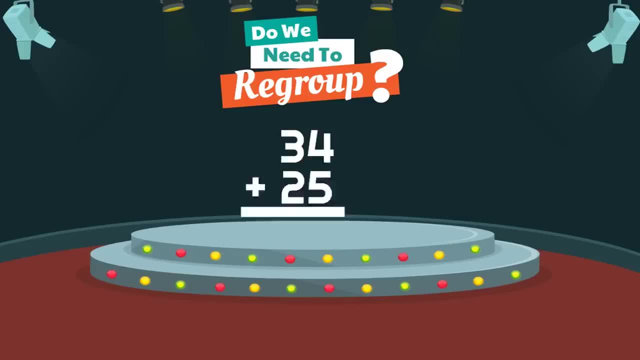 Here is our next one: 34 plus 25.. This is the question: When we add 34 and 25,, do we need to regroup? The answer is no, because 4 plus 5 equals 9.. And 9 is a single-digit number that can fit under the 1s. 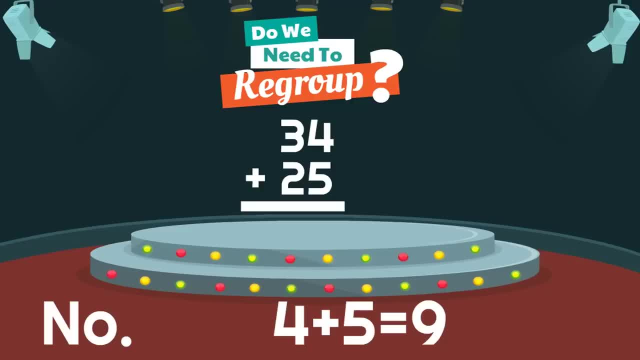 Remember, the first step we take is adding up the 1s, And since the sum is a single-digit number already, we do not need to regroup. Well done, Let's go ahead and finish the problem, just for fun. So when we added up the 1s, our sum was 9.. 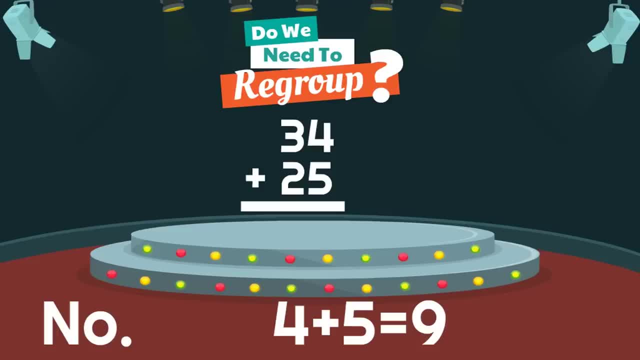 We do not need to regroup. Well done, Okay, we're done, then We're going to go ahead and finish the problem just for fun. So when we added up a single digit number, we were able to regroup 4 and 2.. 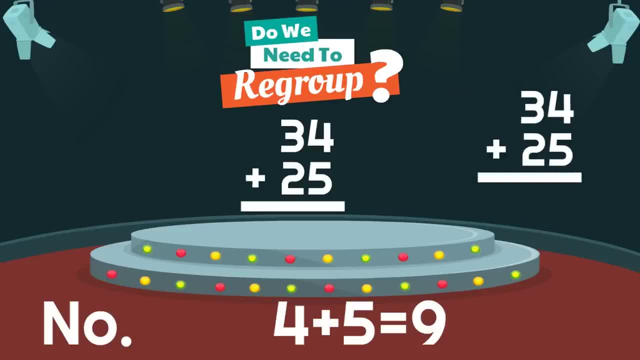 for fun. So when we added up the ones, our sum was 9.. We'll put the 9 under the ones. Then we just add up the tens. What is 3 plus 2?? Uh-huh, 5.. And we have our answer: 34 plus. 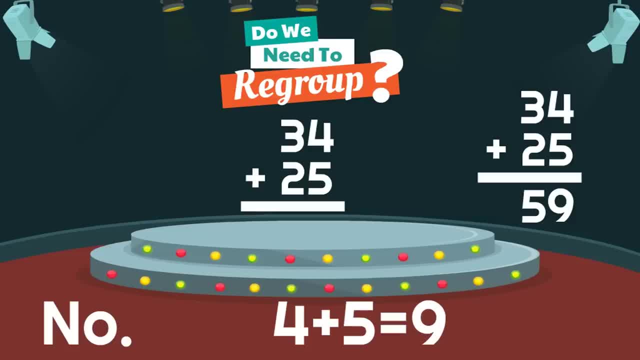 25 equals 59. And no, we did not have to regroup. This is our last one. You have been doing great. 43 plus 37. You already know the question: When we add 43 and 37, do we need to regroup? Yes, because 3 plus 7 equals 10,, which is. 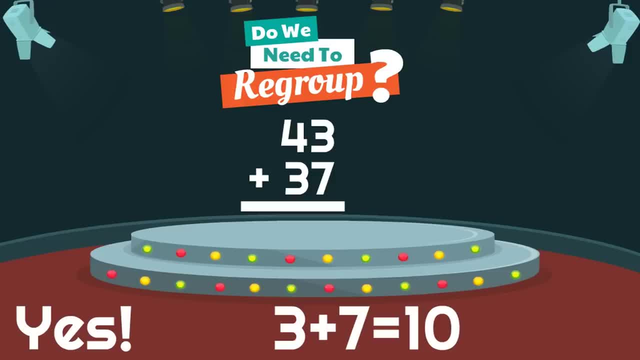 a double-digit number. Remember, the first step we take is adding up the ones, But if the sum is a double-digit number, you have to regroup. That means we need to regroup. Wonderful, Let's go ahead and finish the problem. When we regroup, we split the digits, So the number 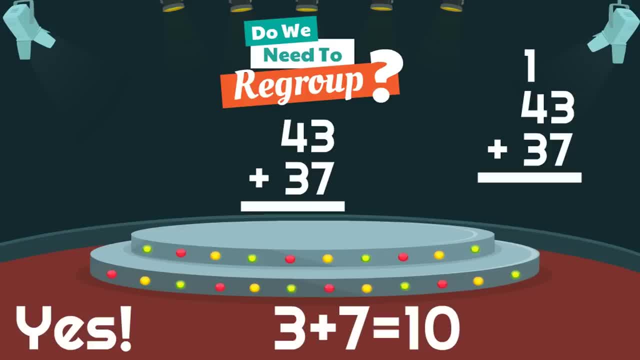 1 gets carried and the second number, in this case the number 0, stays down under the ones. Then we just add up the tens. What is 1 plus 4 plus 3?? Uh-huh, 8.. So 43 plus 37 equals 80.. And yes, we did have to regroup. 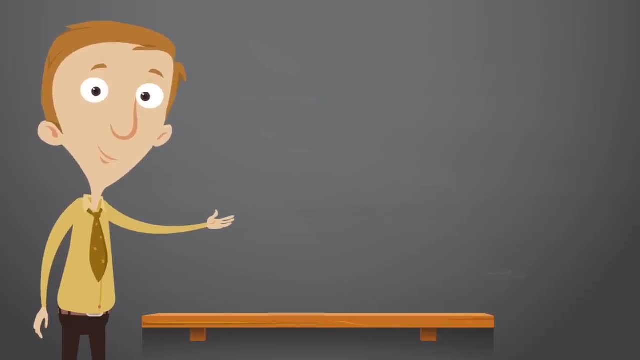 We've had such a great time In this video. we have learned so much about double-digit addition. Two of the biggest things we learned is how it works. We add the ones first- the right side- and then add the tens- the left side. We also learned about something special. 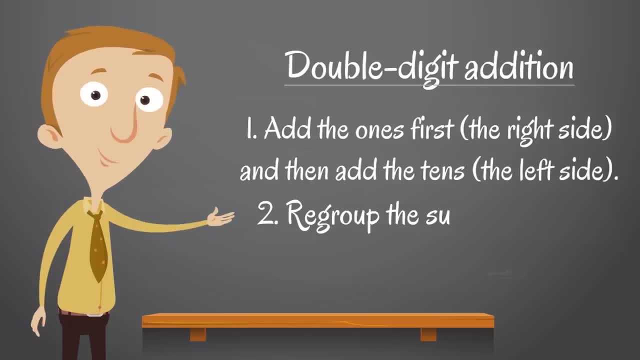 called regrouping And how we need to regroup the sum of a column if it is a double-digit number. 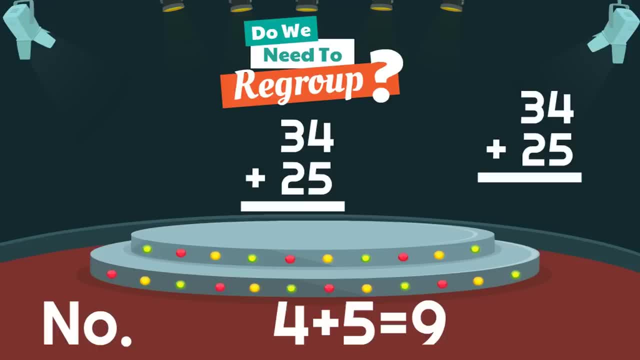 We'll put the 9 under the 1s, Then we just add up the 10s. What is 3 plus 2?? Uh-huh, 5.. And we have our answer: 34 plus 25 equals 59.. 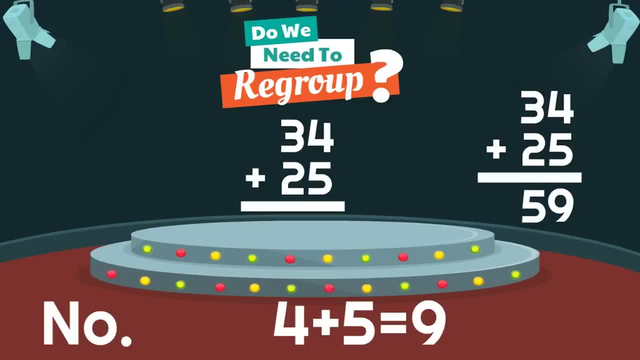 And no, we did not have to regroup. Let's go ahead and finish the problem just for fun. So when we added up the 1s, our sum was 9.. We'll put the 9 under the 1s. 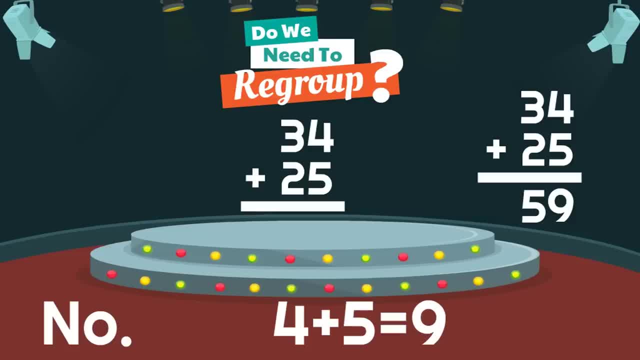 Then we just add up the 10s. What is 3 plus 2?? This is our last one. You have been doing great. 43 plus 37. You already know the question: When we add 43 and 37, do we need to regroup? 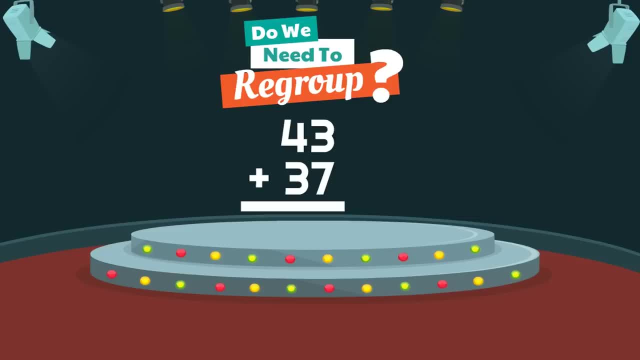 Yes, because 3 plus 7 equals 10,, which is a double-digit number. Remember, the first step we take is adding up the 1s, But if the sum is a double-digit number, that means we need to regroup. 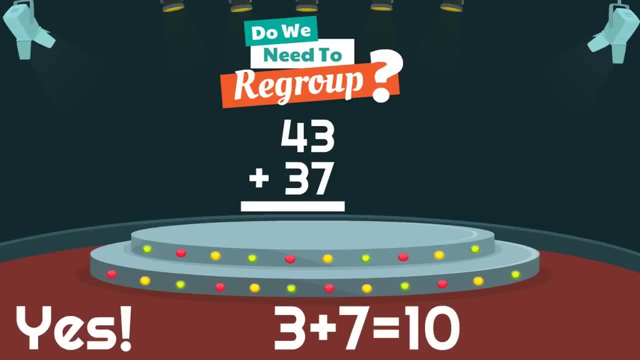 Wonderful. Let's go ahead and finish the problem. When we regroup, we split the digits, So the number 1 gets carried And the second number- in this case the number 0, stays down under the 1s. Then we just add up the 10s. 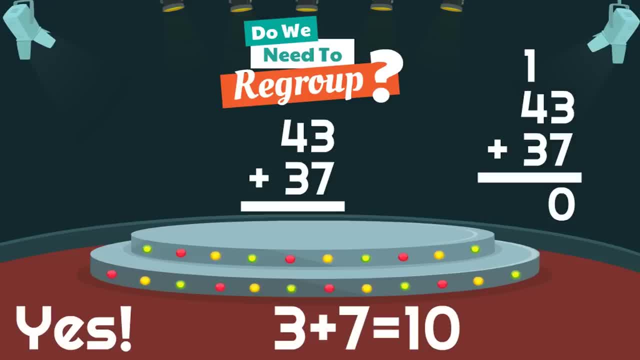 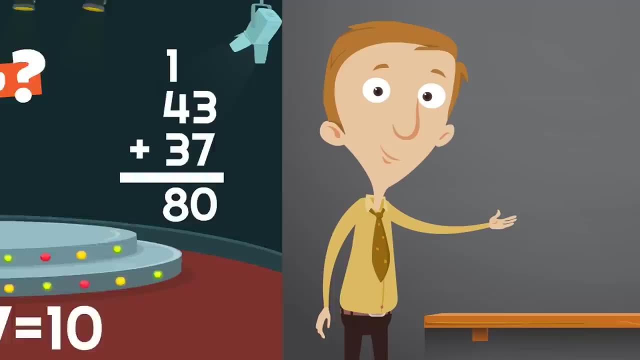 What is 1 plus 4 plus 3?? Uh-huh, 8.. So 43 plus 37 equals 80. And yes, we did have to regroup. We've had such a great time In this video. we have learned so much about double-digit addition. 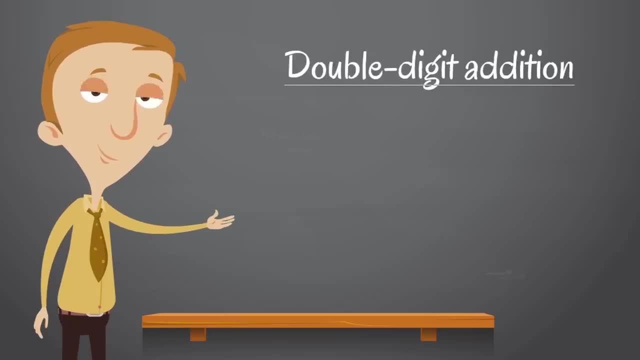 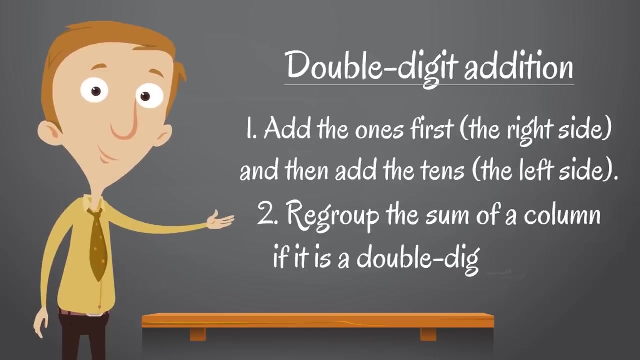 Two of the biggest things we learned is how it works. We add the 1s first, the right side, and then add the 10s- the left side. We also learned about something special called regrouping and how we need to regroup the sum of a column if it is a double-digit number.